So the periodic table of elements is connected to the unknown level of a daily space or establishing 超学, which means the child, a particle of the jumped dish. But remember you can't always do that or you won't be able to solve it in the早 upright context. So when you look at the table, 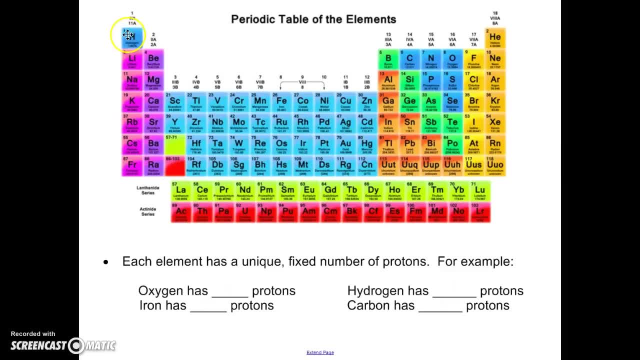 the total intense fault will result in the crucial mart 준비 method, which is what they call the stop-alarm method, And you'll notice that each element, the top left corner, has a number. it's called the atomic number. the atomic number tells you how many protons there are in every. 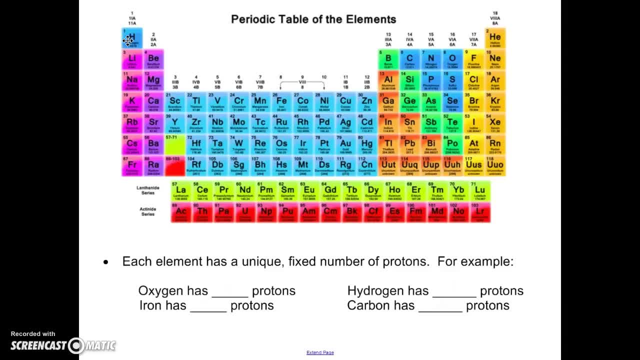 atom of that element and the number of protons for an element is a fixed number, which means it can never change. hydrogen, for example, has an atomic number of one, which means that hydrogen always has one proton it has to oxygen. atomic number is eight. there are always eight protons in oxygen. iron has an atomic number of 26. 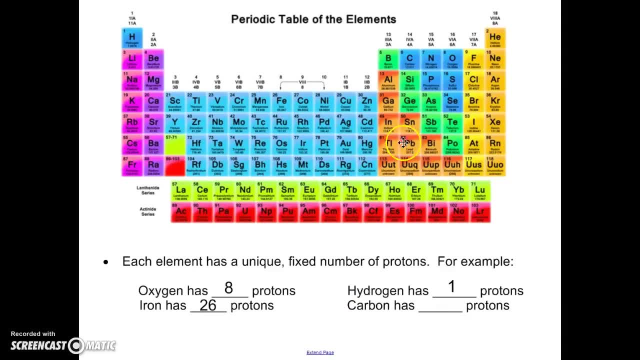 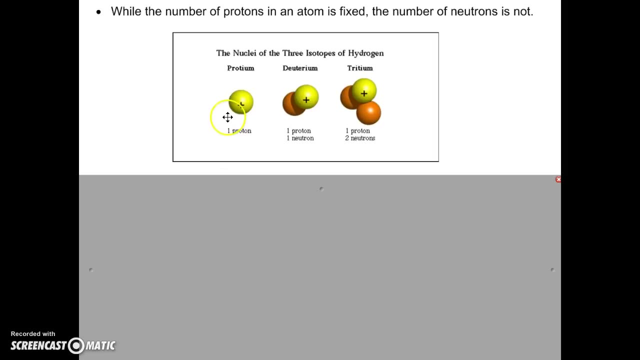 so there are 26 protons and carbon has an atomic number of six, meaning there are six protons in carbon always. now, while the number of protons is fixed, the number of neutrons is not. so here we have three different types of hydrogen. they all have one proton because it's a fixed number of neutrons. it's not a 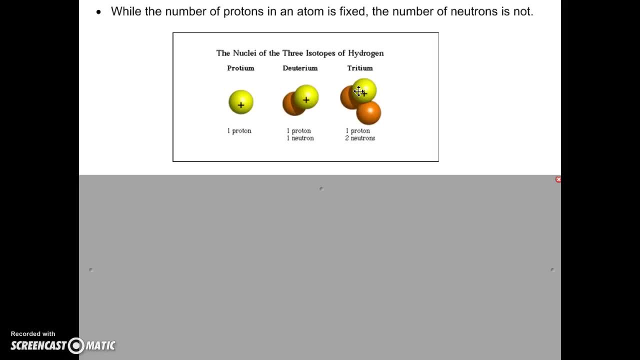 hydrogen has to have one proton. but you'll notice they have different numbers of neutrons. in this first variety there are no neutrons. in this type of hydrogen there's one neutron and in this type there are two neutrons. different varieties of an element are called isotopes. let's look at another. 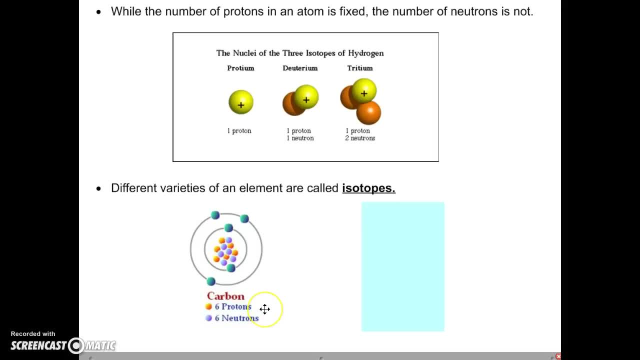 one. let's get carbon. we said before that carbon always has six protons, sometimes neutrons also. but there's another isotope of carbon, there's another variety in which there are eight neutrons. it's still carbon. it's just a different isotope, a different 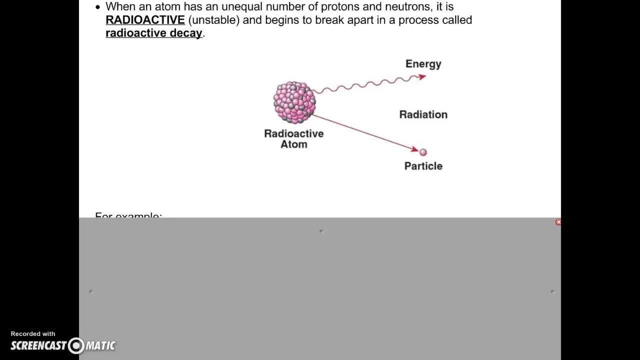 variety of carbon. now the thing is: when atoms have an equal number of protons and neutrons, it's stable. but when the number of protons and neutrons are not equal, the atom is radioactive or unstable. and if an atom is radioactive, it begins to break apart in a process called 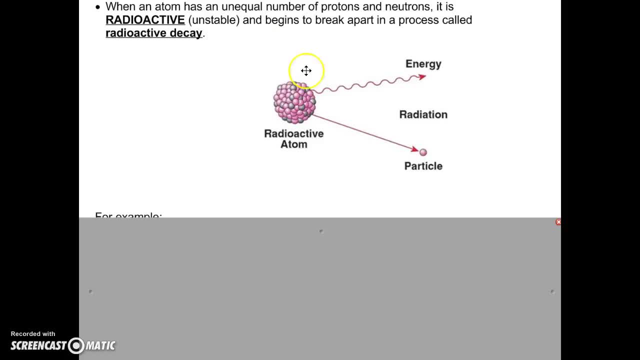 radioactive decay. here's a picture of the process. so we have this unstable radioactive atom. it wants to become stable. it doesn't want to be unstable, so what it will do is it will decay. it will turn into something that is stable and in the process it will release energy. this is nuclear energy. this is how we 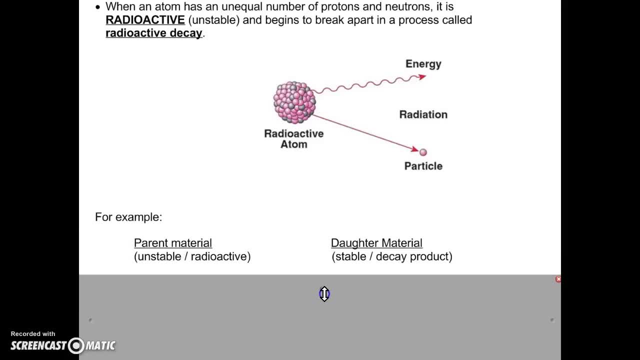 get energy, and this is how we get energy from nuclear power plants, for example, carbon 14. carbon 14 is unstable or radioactive. it will decay into nitrogen 14, which is stable, and we have a lot of different words that we use for these. so the carbon 14, we can call it unstable, we can call it radioactive. we 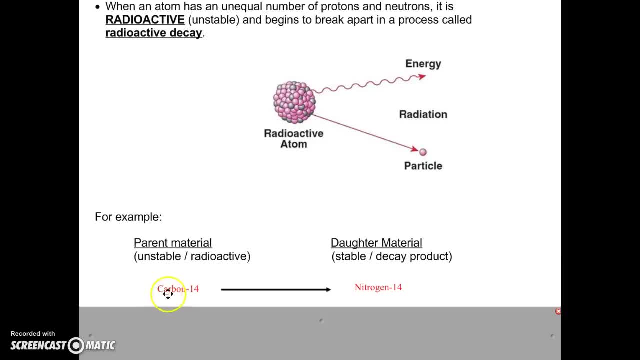 also refer to it as the parent material. the thing that it turns into is called the daughter material or the stable product or the decay product. okay, they're all synonymous. they all mean the same thing. another example: there is a radioactive element called uranium 238. it decays into lead 206, which is stable. on the front page of your earth science reference table. 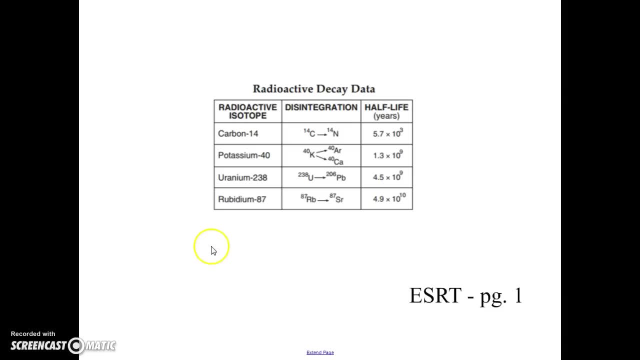 you have this chart that shows you radioactive decay data, and it gives you four different isotopes which are radioactive. it shows you what they disintegrate or decay into, and then they give you something called the half-life, which we'll look at in a minute. actually, let's look at that now. 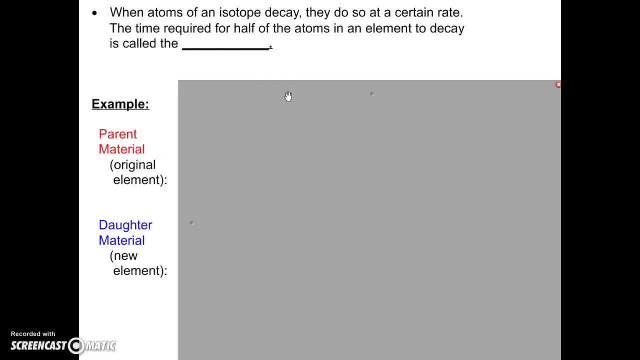 when these radioactive elements decay. the decay happens at a certain rate, certain speed. the time that it takes for half of the atoms to decay is called the half-life. so let's say that an animal just died and the animal has carbon 14 in it. the moment that it dies, all the carbon 14 is still there. a hundred percent of it is there. 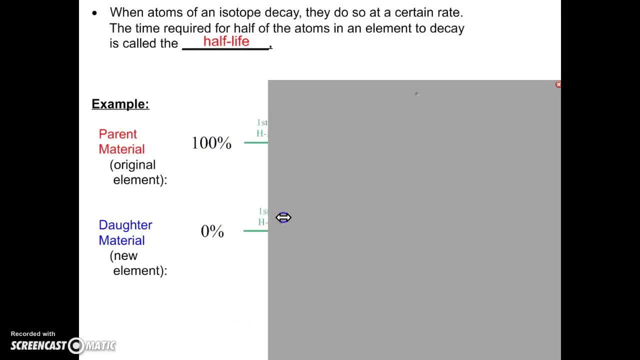 nothing has decayed yet. after one half-life, half of the parent material will decay. so now there's only 50 percent of the parent left and the part that decayed turned into the daughter. when we come up we still will have a hundred percent. after a second half-life we're going to lose another. 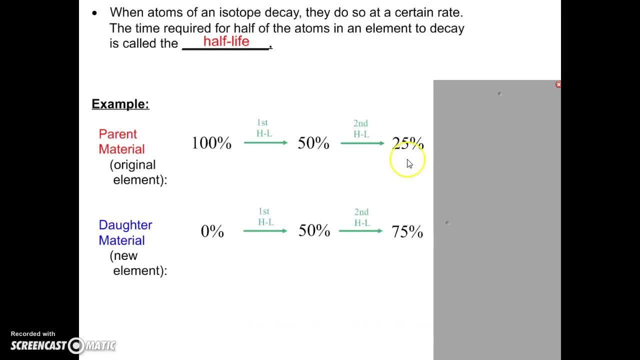 half of the parent. so now there's 25 percent left of the parent and 75 percent of the daughter. it still equals a hundred percent. after a third half-life we're going to lose another half of the parent. so now we only have twelve and a half percent of that parent material left. the rest has. 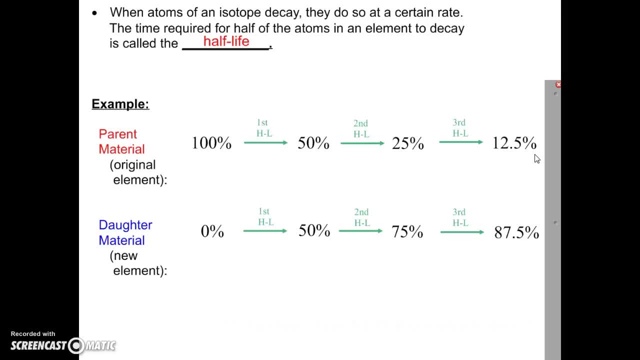 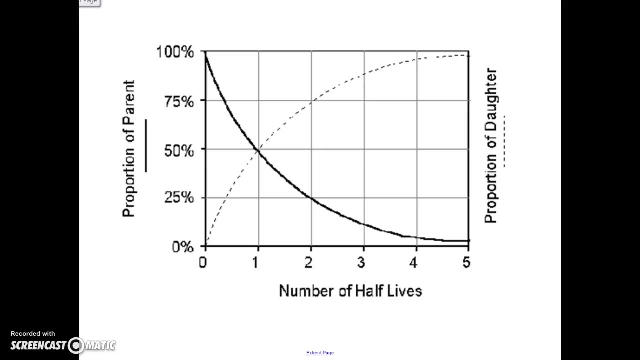 to the daughter, and we could keep going: fourth half-life, a fifth half-life, and so on. we just keep taking away half of what's left of the parent. when you graph this, your graph will always look like this. it doesn't matter which of the isotopes we're talking about. at your zero half-life mark, you're 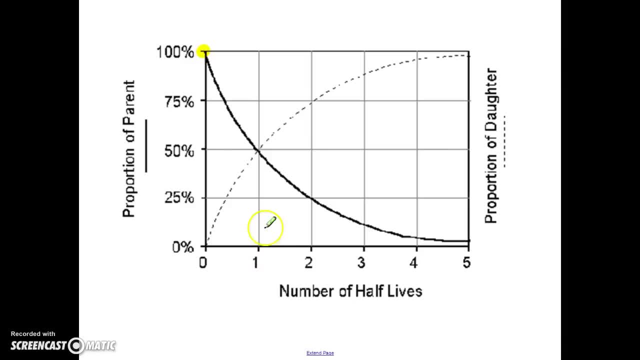 always going to have a hundred percent of the parent. after your first half-life you will have one and fifty percent of the daughter. at your second half-life, you lost half of the parent, so the 50 drops down to 25.. at your third half-life, we lose half of the 25.. we drop down to 12 and a half. 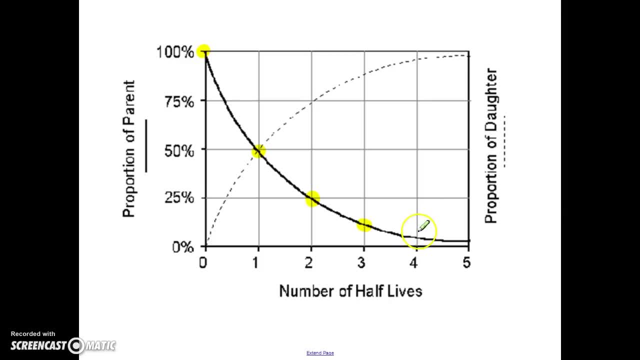 and so on and so forth. now, if you're thinking this through, you hopefully realize that if we keep taking away half, we're never going to get to zero, because if you take away a half and a half and a half and a half, you'll never reach zero. 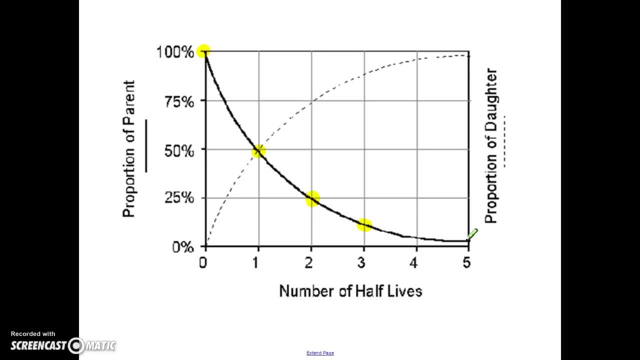 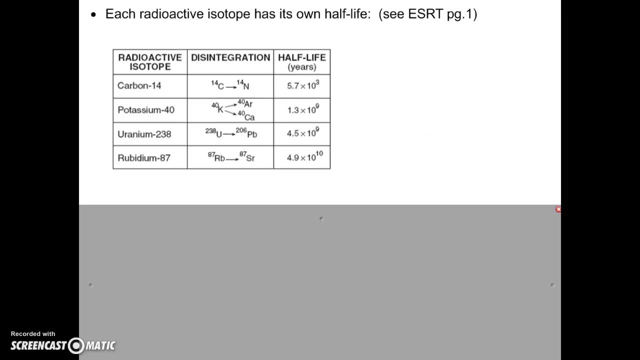 so the parent material will never completely decay and the daughter material will never reach a hundred percent. now every isotope has its own unique half-life. carbon-14 takes five point seven times ten to the third years, or five thousand seven hundred years for half of it to decay. potassium 40 has a 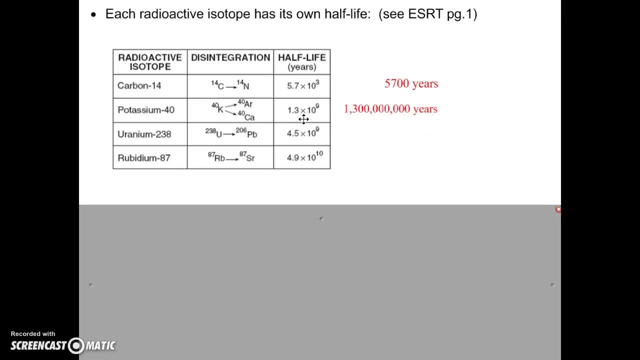 much longer half-life. it takes 1.3 billion years for half of the potassium to decay. uranium four and a half billion years. rubidium: 87- 49 billion years- a huge amount of time. what's key about these half-lives is that half-lives never, ever. 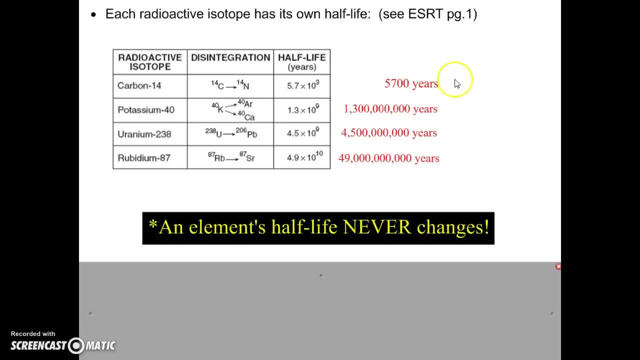 change. carbon-14 will always take five thousand, seven hundred years to go through a half-life. it doesn't matter what you do to it. you can heat it, you can cool it, you can crush it, you can cut it in half. it doesn't matter what you do, the half-life will. 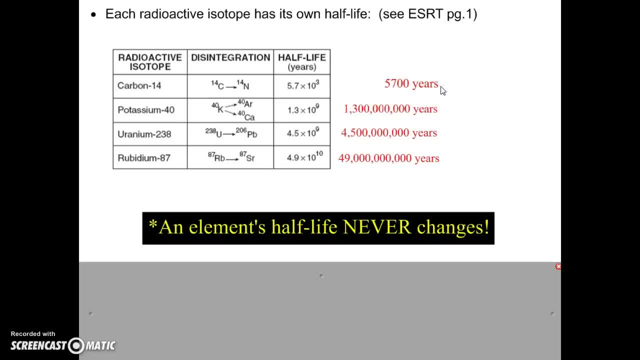 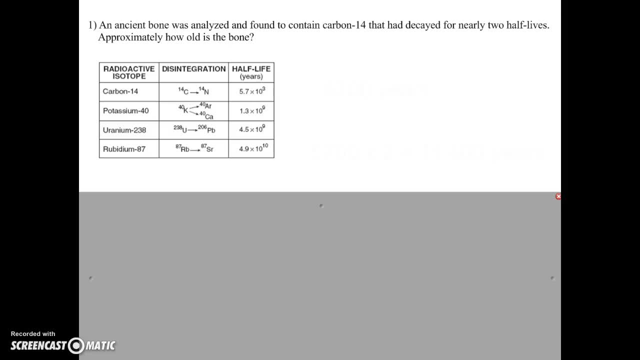 always stay the same, and that is the key to using this process. so let's look at a couple of practice questions. ok, question what: an ancient bone was found and analyzed and found to contain carbon-14 that had decayed for nearly two half-lives. they want to know how old the bone is. ok, well, we know that one. 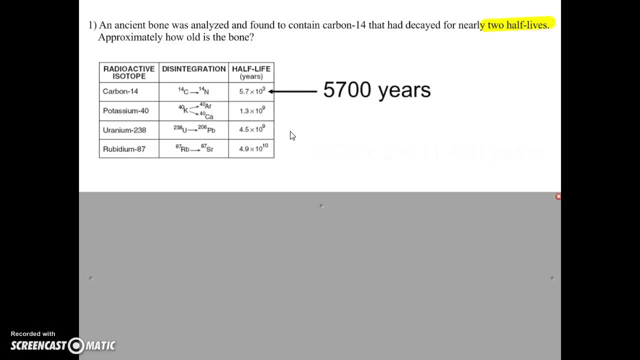 half-life for carbon is five thousand seven hundred years. so if it has gone through two half-lives, it means it went through that two times. so five thousand seven hundred times two is going to equal 11,400 years. let's look at a second problem. 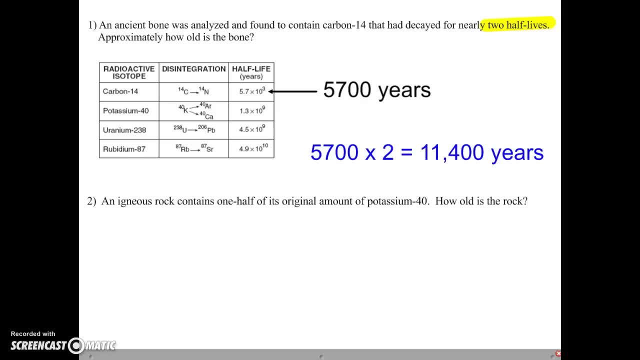 an igneous rock contains one half of its original amount of potassium 40. how old is the rock? ok, so they're telling us that this rock contains one half of what it originally had, so we're going to refer back to that chart that we looked at before this. 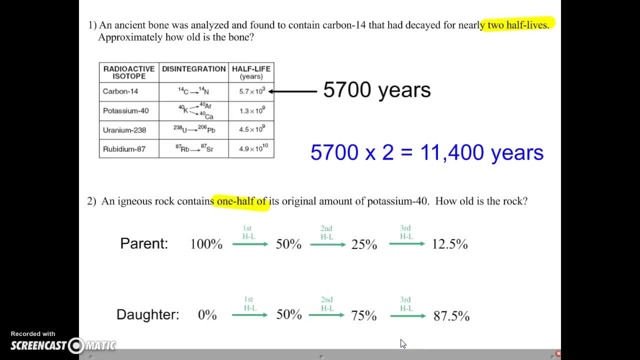 chart will help you with any of these questions. my advice is to always draw this out on your paper and then use it for as many questions as you need to. ok, so the rock has 50% of its potassium 40, so we know we started off with a. 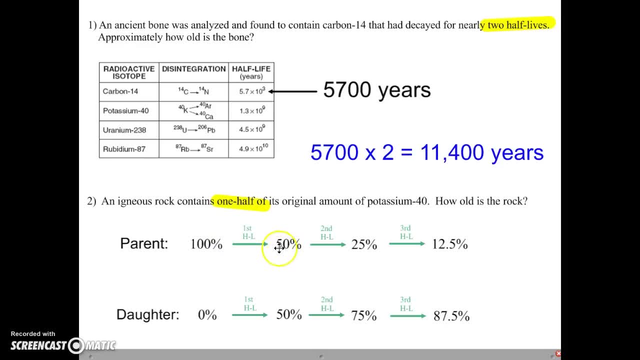 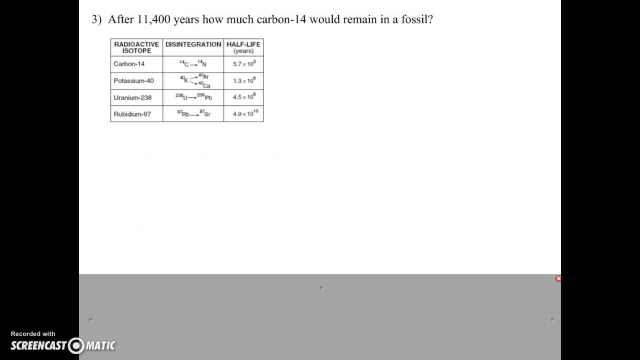 hundred percent, and if I'm left with 50%, that means it only went through one half-life. so for potassium 41 half-life is 1.3 billion years. so that's how old this rock would be. so get another one after 11,400 years. how much carbon-14. 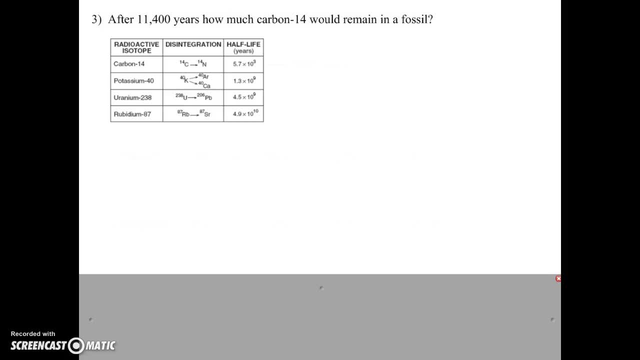 would remain in the rock. ok, so now they're giving us a longer amount of time and we have to determine when this fossil died and how much carbon-14 would be remaining. so we know that the half-life for carbon-14 is five thousand seven hundred years. 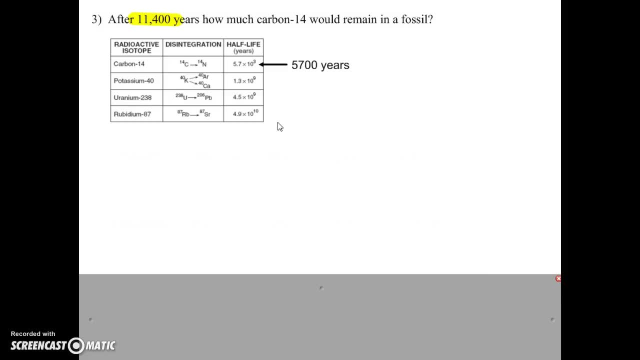 that's how long it takes for half of the carbon to decay. we have to figure out how many half-lives would go into this total amount of time. so it turns out for this problem that if you multiply 5700 by two you will get 11,400. so this is going to be equal to two half-lives. so again, we're going to 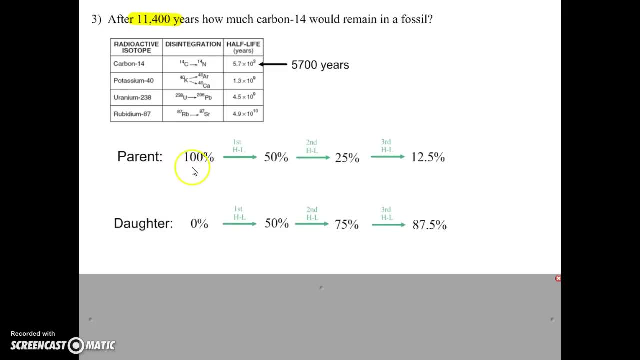 want to use that same chart. so we started with a hundred percent after the first half-life were down to 50, after the second half-life were down to 25. so the answer for this question is there would be twenty-five percent of the carbon-14. 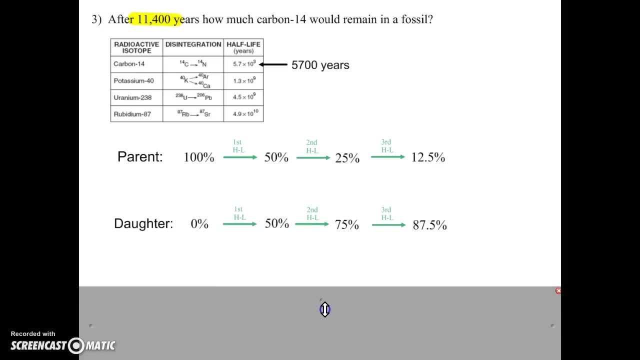 left alright. question four: if radioactive material were cut into pieces, what would the half-life of each piece be? so do you remember what we talked about before right? half-life never changes. it doesn't matter if you cut it into pieces, it's going to be the same. 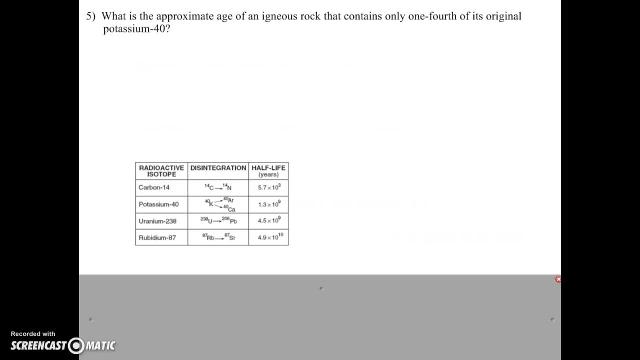 ok, let's look at two more questions. so what is the approximate age of an igneous rock that contains only one rock- I'm sorry that we're sitting on a Doать channel- and number three has to be about one-fourth of its original potassium-40. so there's only one-fourth of it remaining, so that's the key to. 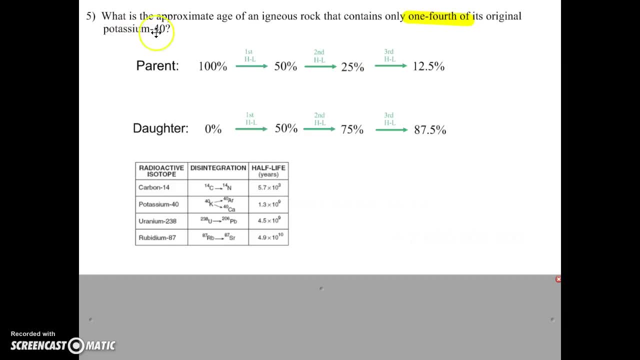 figuring this out. so again, I need that chart. well, if there's only one-fourth left, that means it went through two half-lives, because two half-lives gets. Now we said it had to go through two half-lives, so we're going to simply multiply this by two. 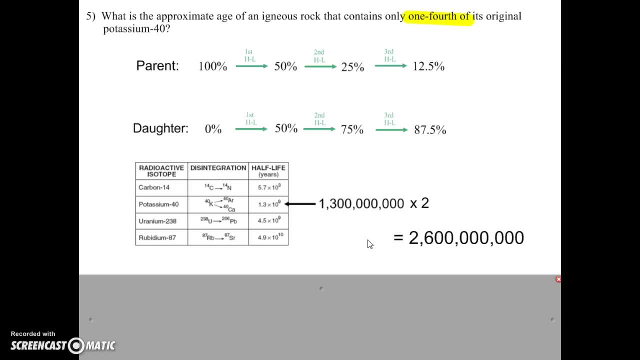 and that will give us 2.6 billion years. That's the age of this rock. And for the last practice question, a sample of wood found in an ancient tomb contains 25% of its original carbon-14.. What is the approximate age of this wood sample? Okay, so it has 25%, So I come back up to this. 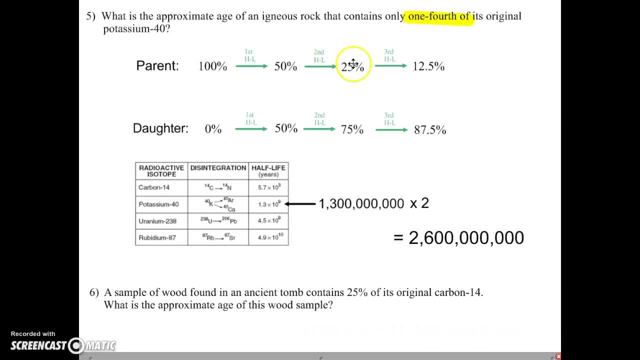 chart. So 25% again, that's two half-lives. Well, I know, for carbon-14, each half-life is 5,700 years. If there have been two half-lives, it means this piece of wood is 11,400 years old. 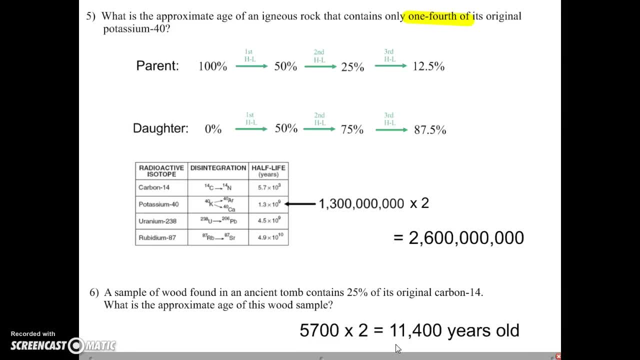 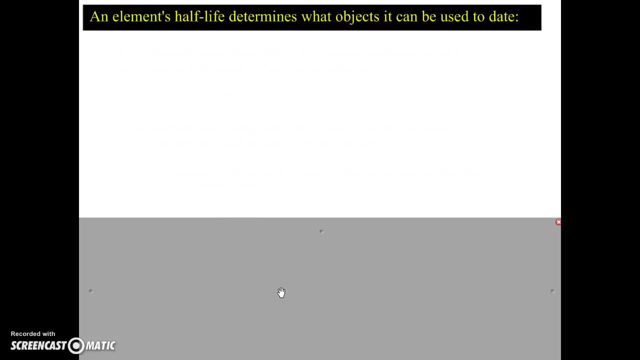 Okay, so those were some practice questions. We'll be doing many more in class. Now there are some other things that you need to be aware of when we're using this process. First of all, if you want to use this process, you need to be aware of the fact that it's a process. So, if you want to, 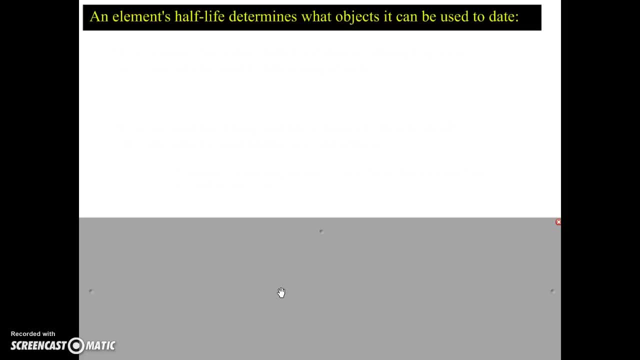 use this process, you need to be aware of the fact that it's a process. So if you want to use this process, you need to be aware of the fact that it's a process. So if you want to use this technique, you have to figure out which element to use. If an element has a short half-life, it means that 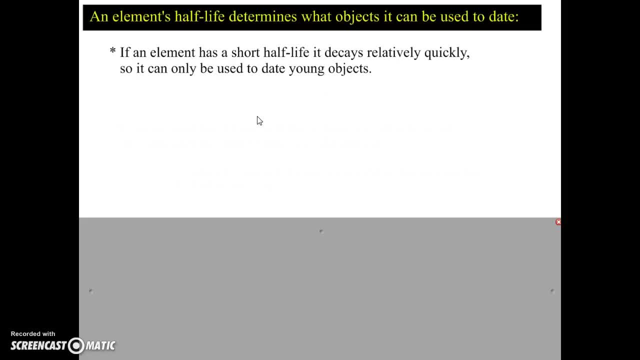 it breaks apart quickly, And so after a short amount of time it will have broken apart so much it's going to be really hard to measure. There's going to be so little of it left. For example, out of the isotopes we've been looking at, carbon-14 has the shortest half-life right. 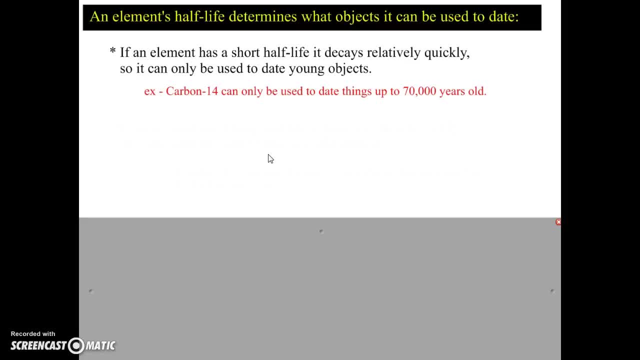 5,700 years. After around 70,000 years, there's not going to be enough carbon left to even measure, So you can only use carbon-14 for things that are not very old If you want to date something that is very. 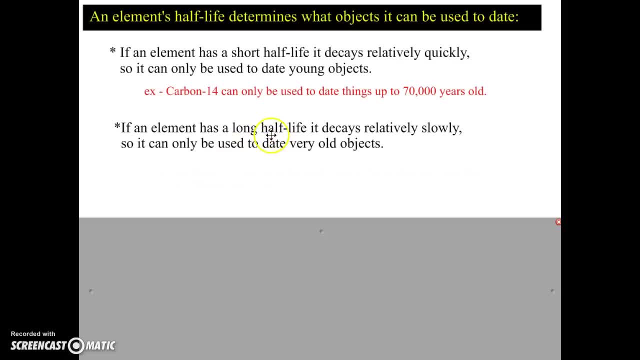 old, then you want to choose an element that has a long half-life. For example, uranium-238 has a half-life of four and a half billion years. That's a long half-life. So if you want to use this technique, you have to think about whether you want an element with a short half-life or a long half-life. 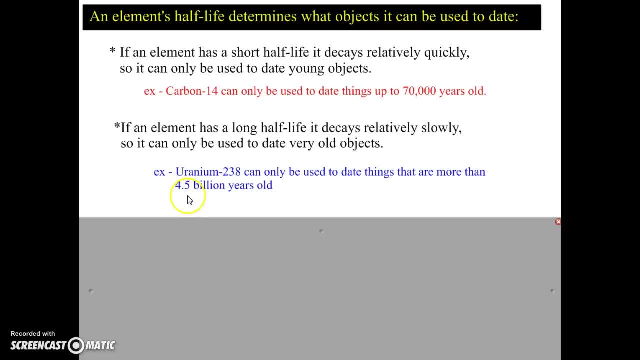 So that means if you have a rock that formed a thousand years ago, you would not be able to use uranium-238 because it did not go through any half-lives yet. right? It takes four and a half billion years to go through one half-life, So the rock would have to be older than four and a half.